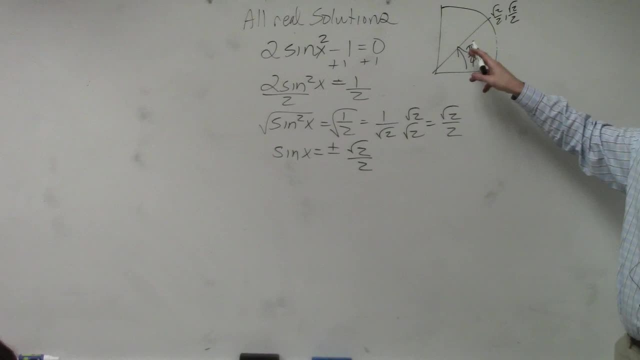 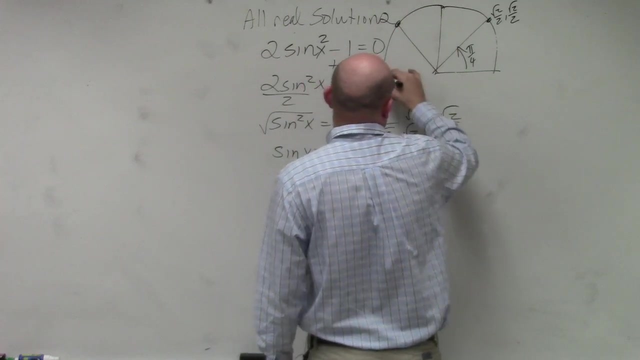 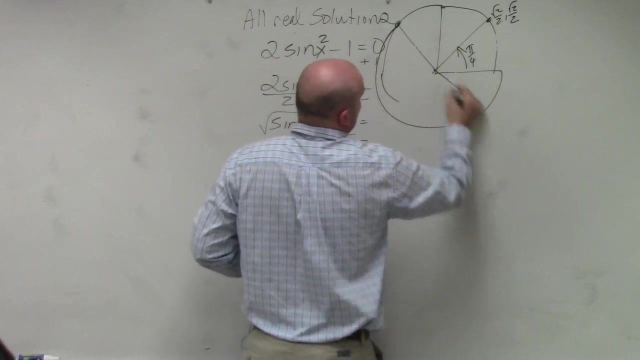 Right. However, is that the only time where we're going to have square root of 2 over 2? No, we basically have the angle over here. I'm going to erase this. You have this angle and you have that angle. 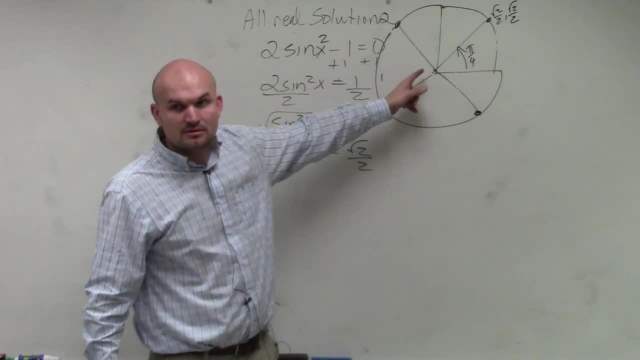 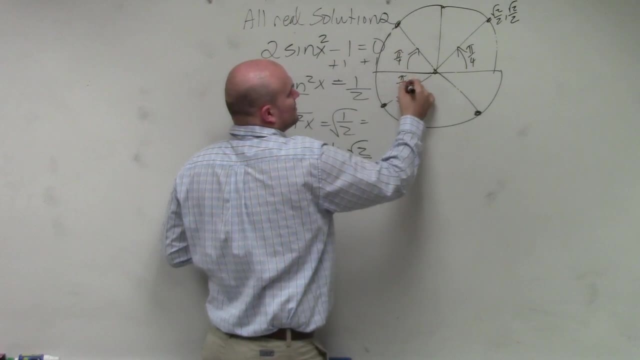 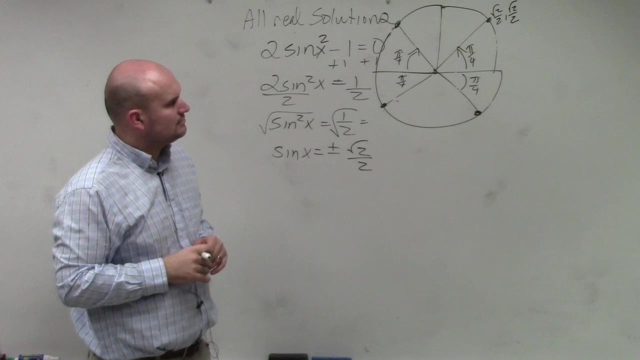 Do you guys agree with me? Those are all like my pi's: Pi over 4's. Yes, It's okay. So all my reference angles are pi over 4.. All the reference angles are pi over 4.. There you go. 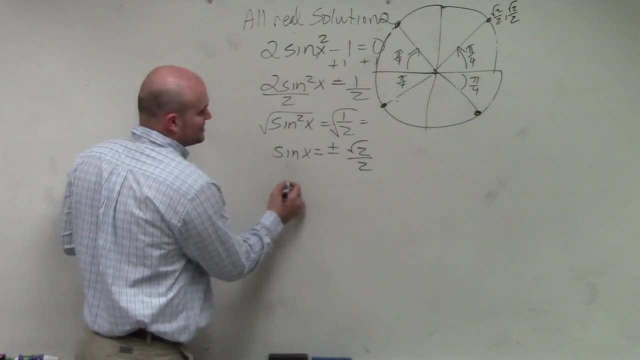 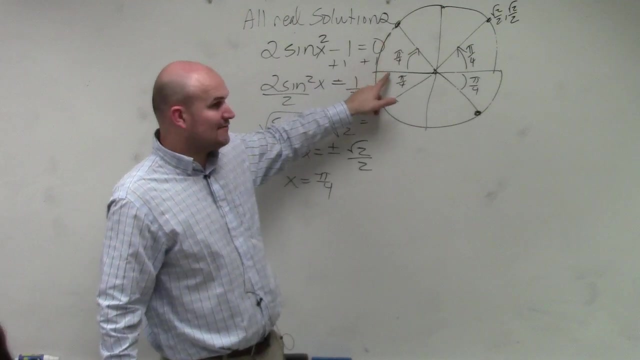 Now. so I know that one of my solutions is x equals pi over 4.. Correct. The next solution. Well, we know, halfway around a circle is pi over 4, or 4 pi over 4.. So if I'm a short one, then I'm at 3 pi over 4.. 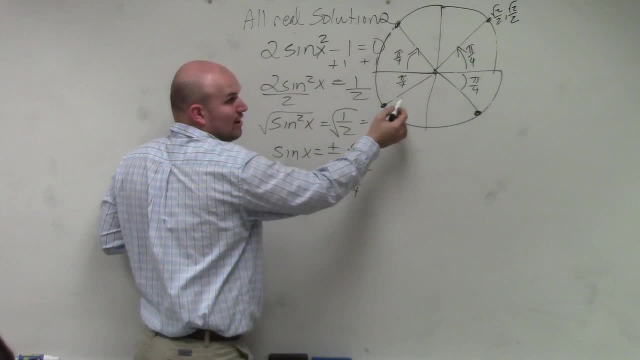 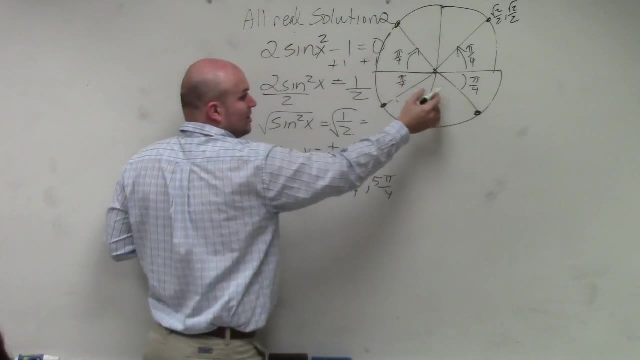 Halfway around a circle is 4 pi over 4.. If I go an extra pi over 4, I'm at 5 pi over 4.. If all the way around the circle is 8 pi over 4, but I'm one short, then I'm at 7 pi over 4.. 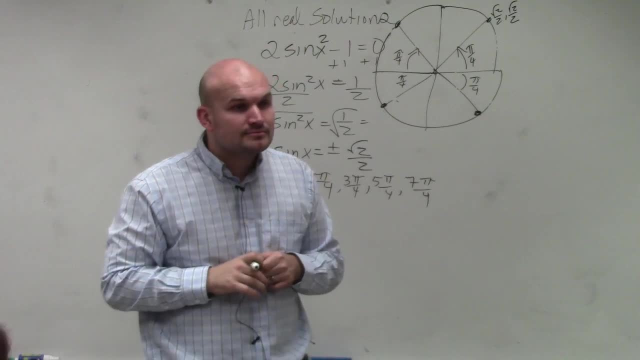 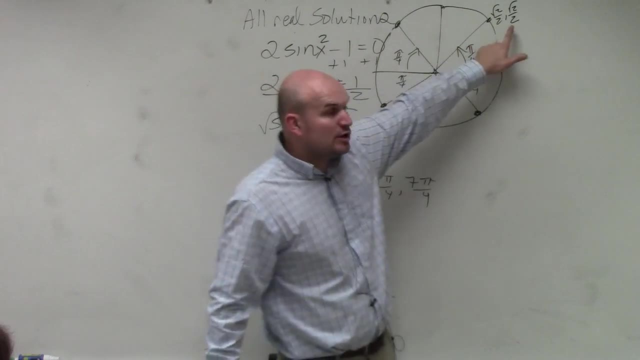 Okay, Now here's where it's going to get difficult. Yes, So are we looking at, like, the angle between each? We're looking for all the angles where the sine is equal to either positive square root of 2 over 2, or negative square root of 2 over 2.. 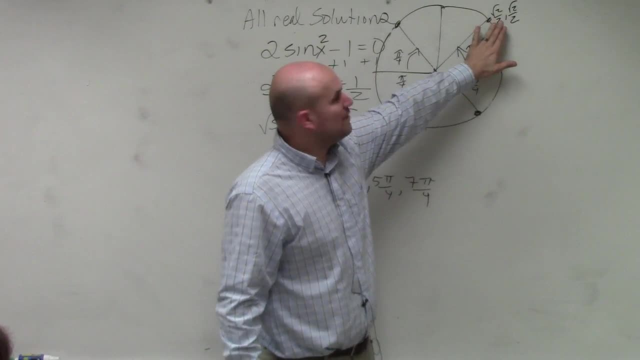 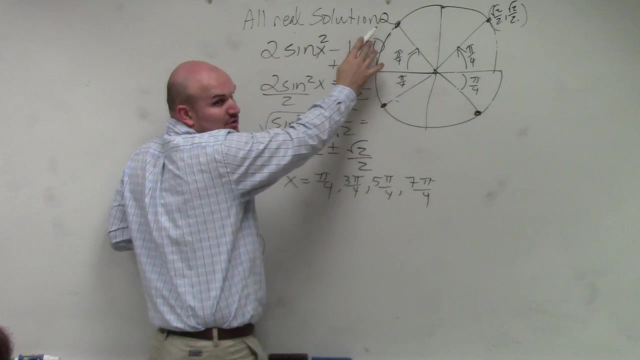 And what I did is, once I found this angle, do you agree with me that if I reflected this coordinate point across the y-axis, the only thing that's going to change is the x-coordinate would be negative. square root of 2, right. 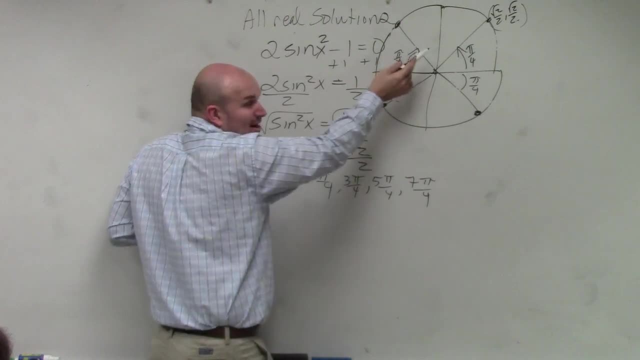 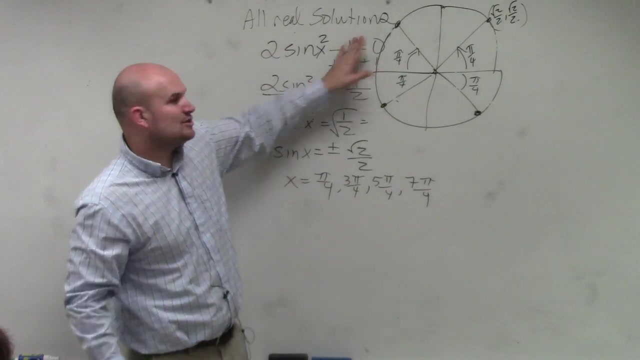 If I reflected over the y-axis, the point is exactly the same, except they're both negative. Do you see that? See what I'm saying. So that gives you all the angles. Now, if my, If my answer was between 0 and 2 pi, I would be done. 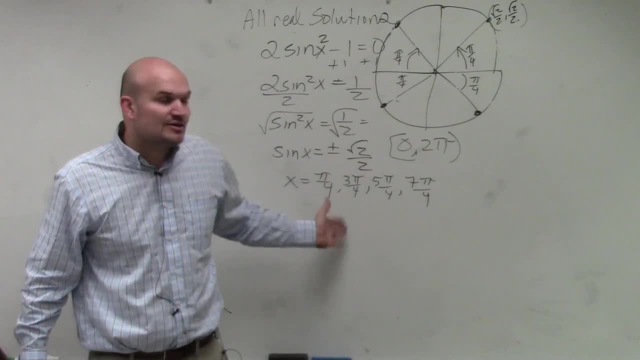 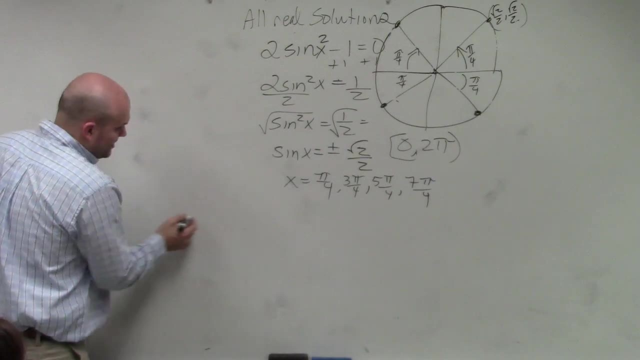 That's what you do Done. However, I'm not asking- They're not asking- for all the solutions between 0 and 2 pi. They're asking for all of the solutions. So what we need to kind of remember here is sine. 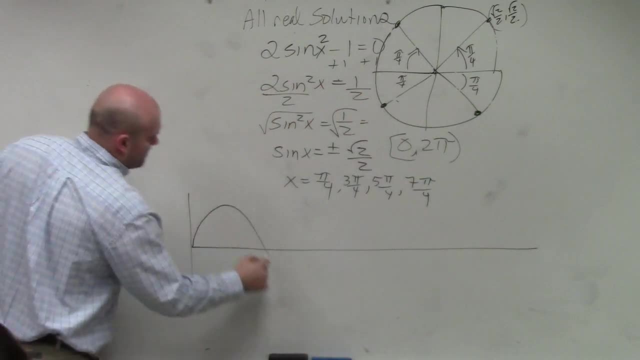 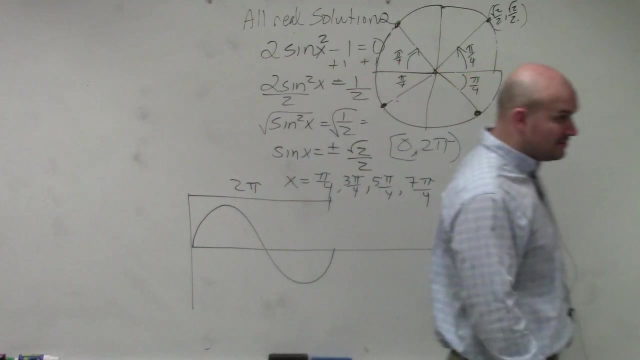 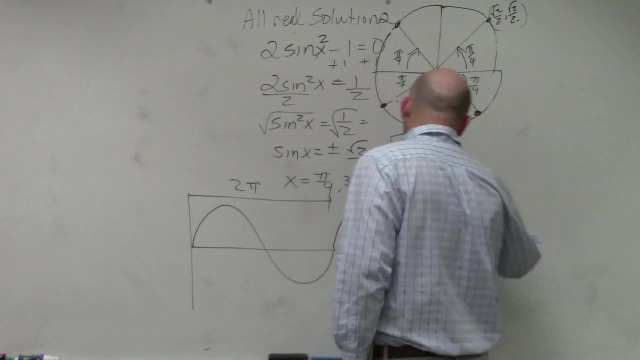 What does sine look like? Here is between 0 and 2 pi, Correct, Correct, So basically. So the first period is like the unit circle, But as you guys remember from graphing, sine goes on and on and on forever. 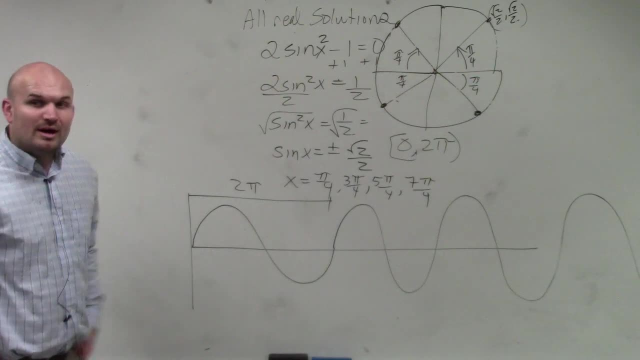 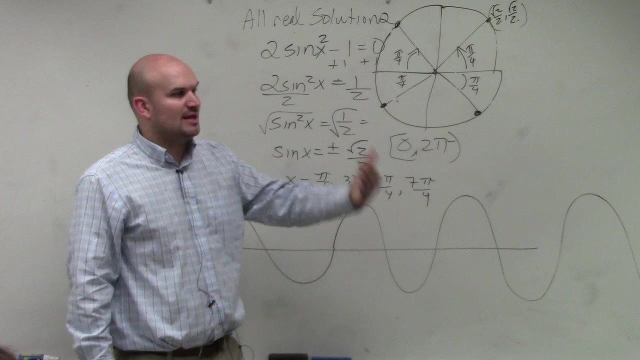 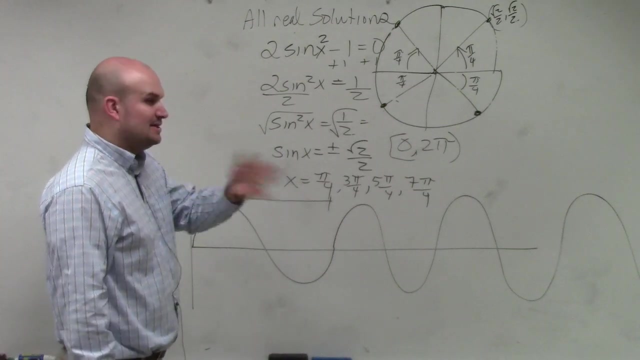 It's never going to stop. So what that means is we need to write our solutions using a variable that can represent infinite many coterminal angles. Well, so here's how it kind of goes, And it's tricky and it's different for everyone. 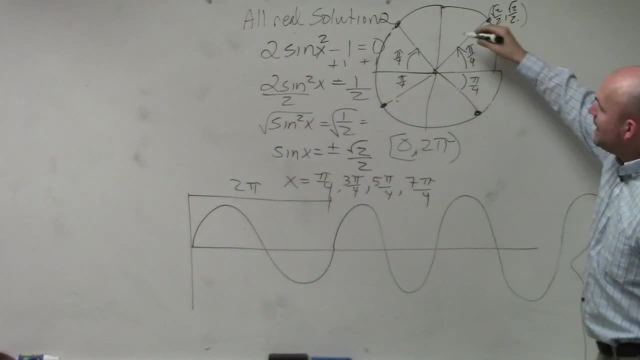 If here's my first answer, here's my first solution. right, Pi, Pi over 4.. How far is it to my next solution? Be careful, How far is that? What is that distance? What is That? looks like 90 degrees, right. 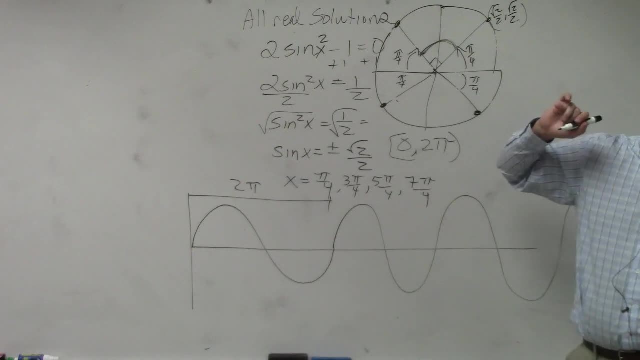 Isn't that pretty close to 90 degrees? Which would be what in radians? Pi over 2.. And then, to get to the next answer, I'd have to do what? Pi over 2.. Pi over 2.. Next one: 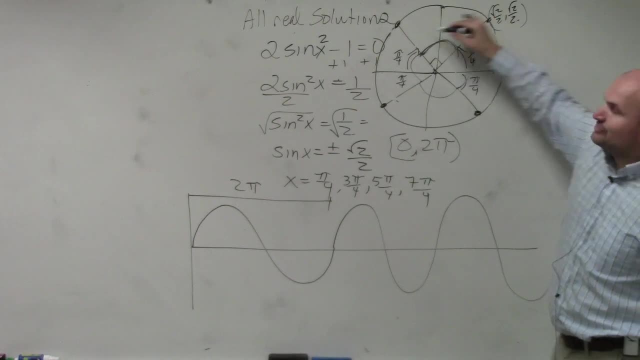 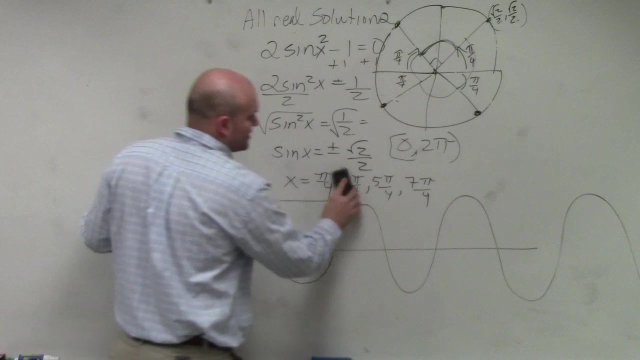 Pi over 2.. Next one: Pi over 2.. Do you guys kind of see how this would keep on going Pi over 2?. So therefore, instead of writing out all the answers, all I can simply do is start with one answer and say: plus, pi over 2 n. 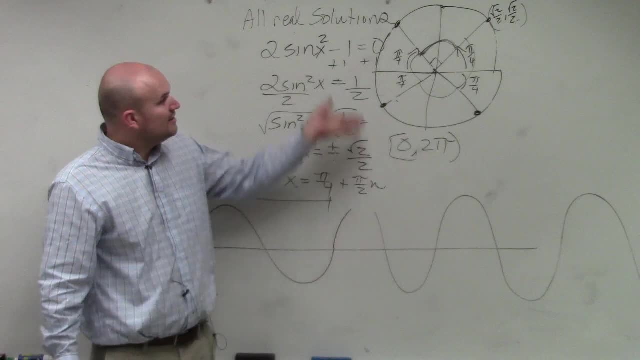 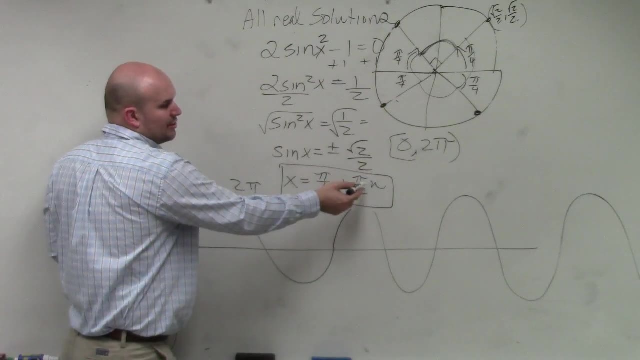 Remember how we wrote asymptotes with n. We're going to do the same thing. So if it's saying, find all real solutions, a lot of times you're going to be using a multiplier n, Pi over 2 n, Instead of just listing the answers. 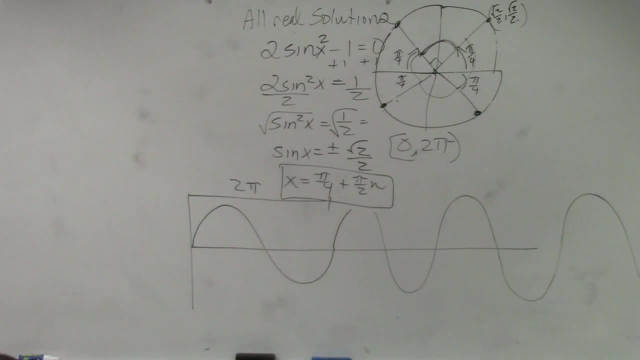 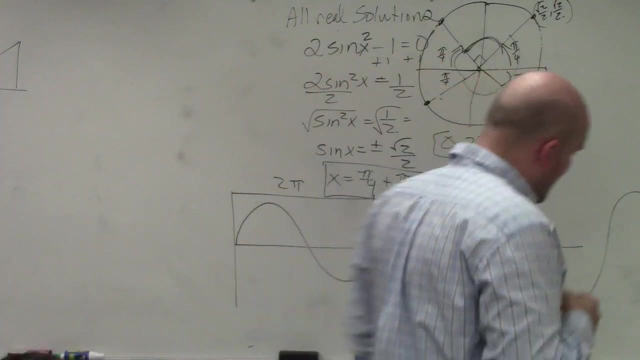 Okay, All right, That's two answers for you. First half is you're finding the answer between 0 and 2 pi. Second half, you're finding all real solutions. Please, guys, it's really hard to learn this stuff unless you're practicing it. 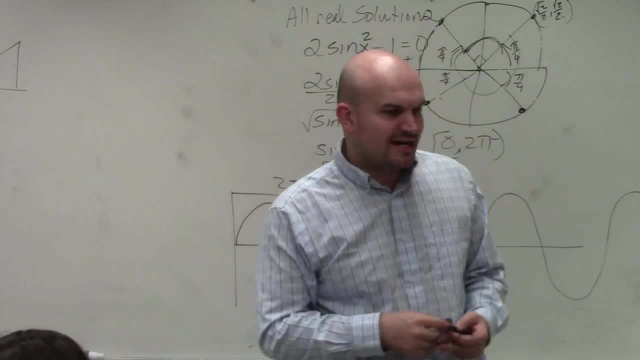 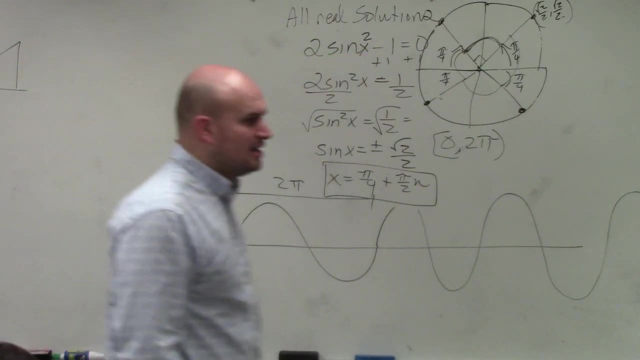 I'll walk around and check your homework. I'm going to also take a picture of something I'm going to show you how to hold And your constraints. We're going to talk about that later. Come around and check out what you're doing. And if you're not going to do this, I'm going to show you how to do it. So I'm going to show you how to do it. So I'm going to show you how to do it. And if you're not going to do this, I'm going to show you how to do it.